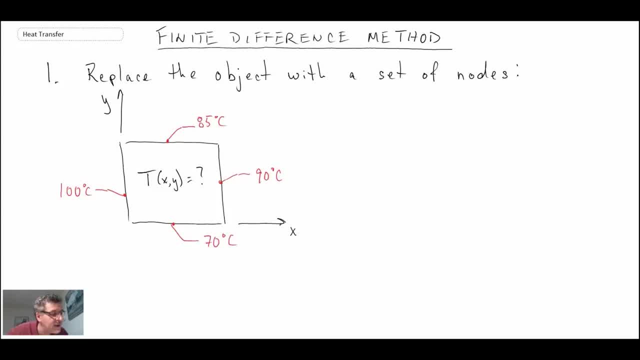 So there we have a plate with four different boundary conditions, one on each side, And this is the problem of a square plate. And then what we want to do? we want to convert that object into a grid of finite nodes. So we would recast that. 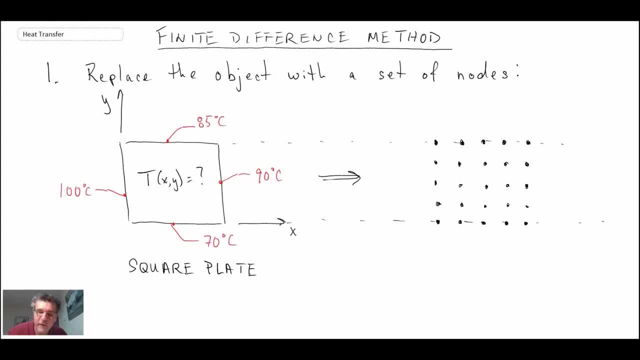 So what we've done is we have represented our square plate through a series of grid points. And then what we would do? we are not going to develop an identity algorithm at this point, but I'd like to show that what we do is we have these two vectors. 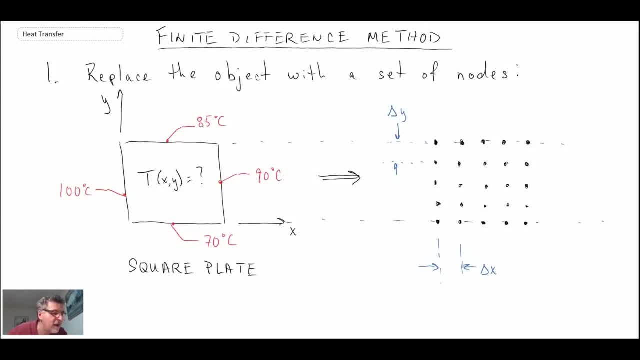 where we have two, three 0s and one 1 0s, And then, given that the velocity of this particular vector, we could apply the footing function. How do we do that? ohh well, we ninth, we can do that for the first one. 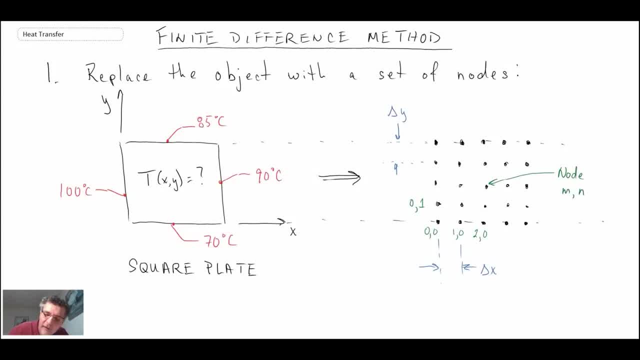 And therefore, as I just did, there are only three vectors in the非. So if I could find the next Nt vector, we would carry Prism-Z today, and then I can occupy this number with the gradient. THEN Now, what we are doing here is we are we're going to group them, placed up here. 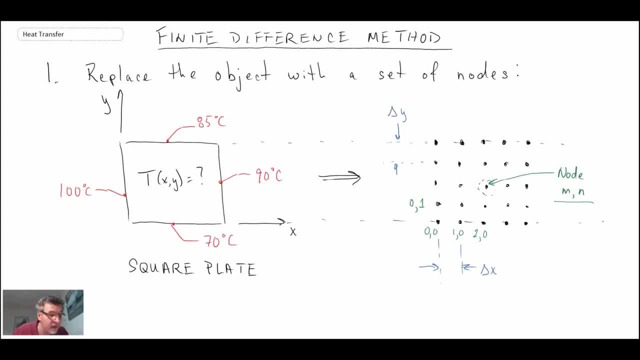 You have- and it seems like this is a nice little queens now- how the nodes relate to the equation in a moment, And so this process in any finite difference technique is referred to as being grid generation. The next step in the finite difference method applied to the heat diffusion equation. 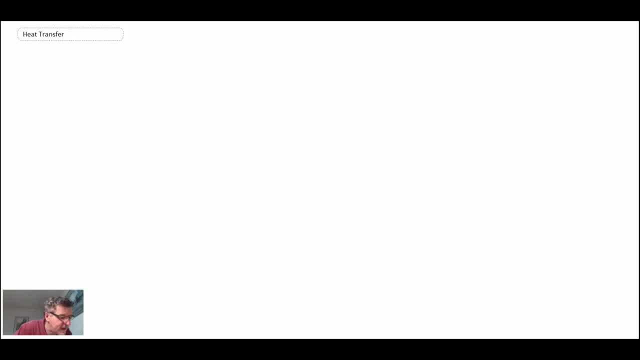 is to rewrite the mathematical physics equation in finite difference form. So if we have a case of a steady heat transfer in two dimensions with internal generation, the heat diffusion equation and partial differential equation would look like this. Now, what we want to do is we want to be able to express that. 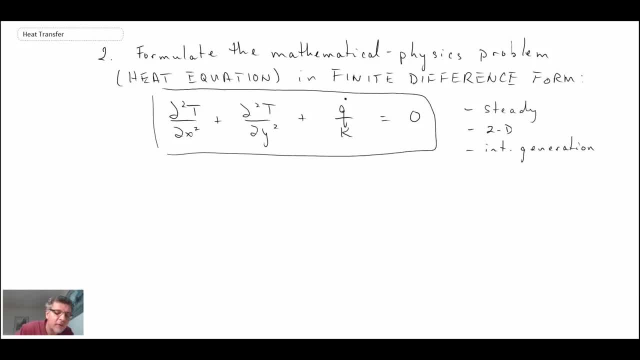 in finite difference form And so, going through a process that I will get into in the next lecture, the following would result: So that's what the finite difference equation, or version of the heat diffusion equation, would be transformed into, And the T, m, n in these equations here. so there and there that refers to: 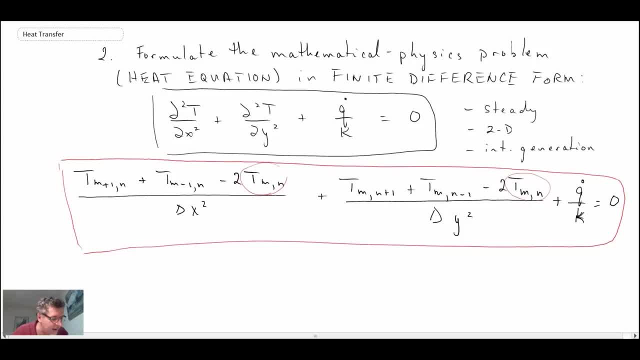 the temperature at nodal location m, comma n And the m? n subscripts are basically just a bookkeeping approach that we use in order to keep track of the temperatures at different points within our grid that we generate in the first step. So that is the second step. You recast your. 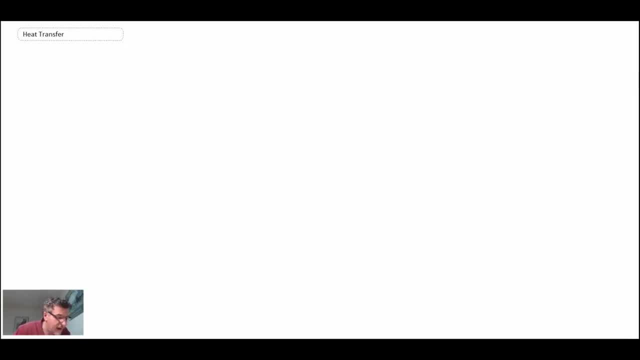 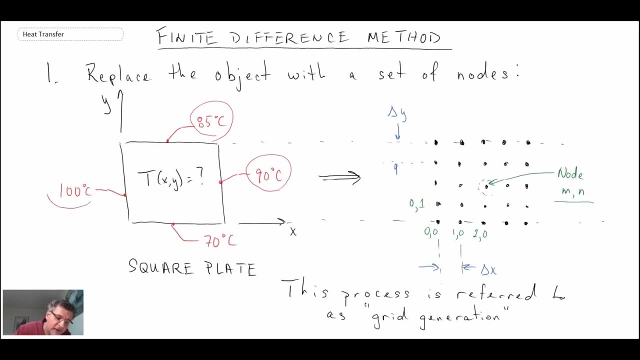 mathematical physics equation. The third step is to figure out how to handle your boundary conditions. So, looking back at the plate that we're trying to solve, our boundary conditions are here And we can see what is specified for this particular problem is a specific temperature along each of the walls of the plate. 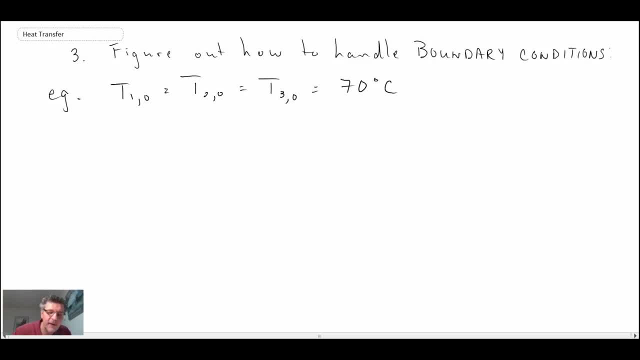 So an example for one of the boundary conditions could be the temperature at nodal location. one comma zero equals two comma zero equals three comma zero equals 70 degrees C, And so that would be an example of how you would handle the boundary conditions on one of the sides. and the last thing that we do in this process: 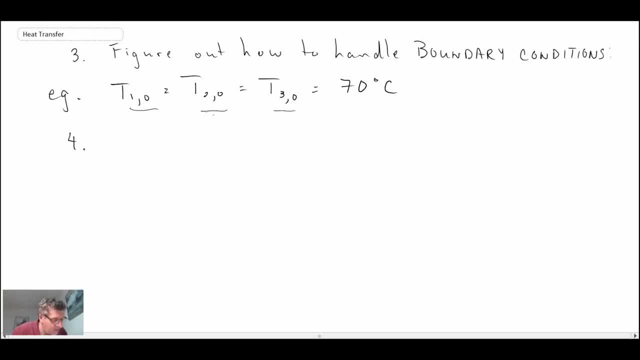 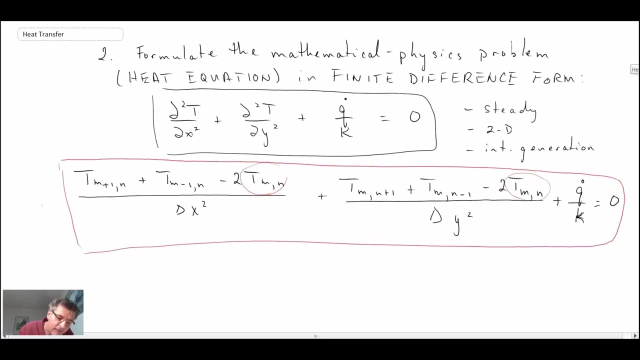 is, we need a way to be able to solve for the temperature distribution, and the way that we do that is the following. so what you do is you apply the finite difference, the equation, the one that we came up with here. so this is the finite difference, the equation, the finite difference, form of our mathematical 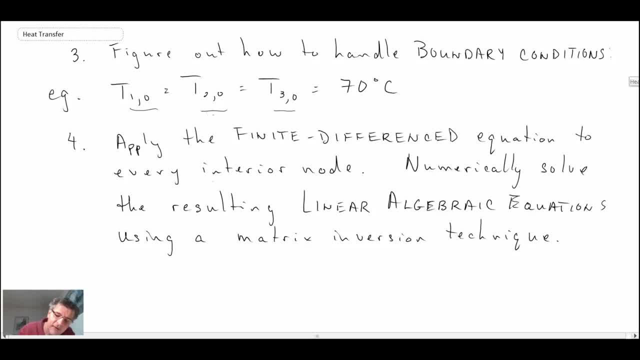 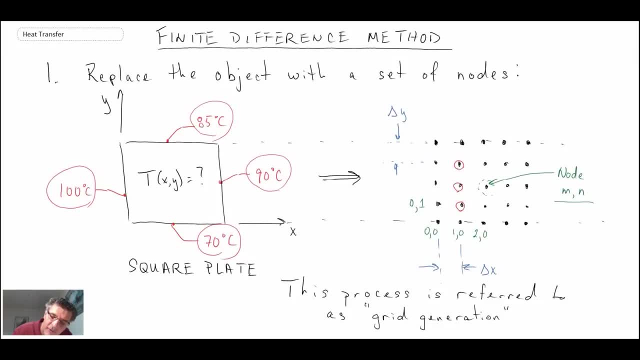 physics equation. you apply that to every interior node. so looking back at our grid, that would be all of the interior node'soring locations. you apply the finite difference, the equation. the external surfaces have all had the boundary conditions applied there. now the corners you got to be a little careful with because the boundary conditions are. 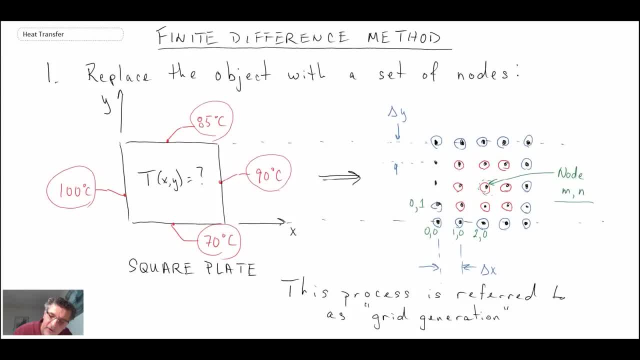 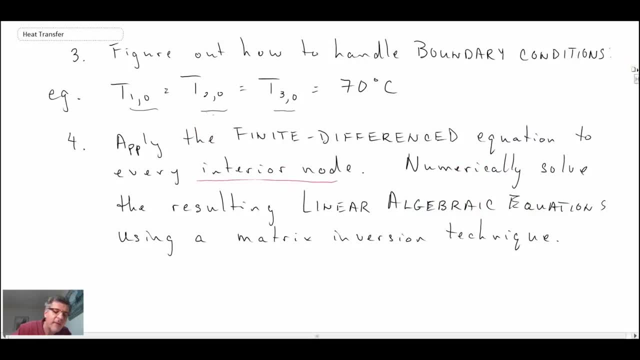 going to be essentially an average of what's going on on each of the walls, but those ones have been handled by the boundary conditions. it's the interior nodes that we're going to apply the mathematical physics equation to, and that is going to result in a linear, a series of linear algebraic equations. 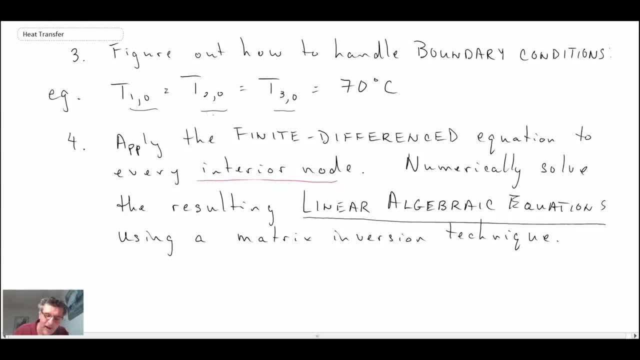 that you need to solve with some technique and essentially you're using a matrix inversion technique. and if you look in numerical methods textbooks, there are different methods of doing matrix inversion for linear algebraic equations and one is the Gauss Jordan elimination technique and this is a direct method. another one is the Gauss Seidel technique and this 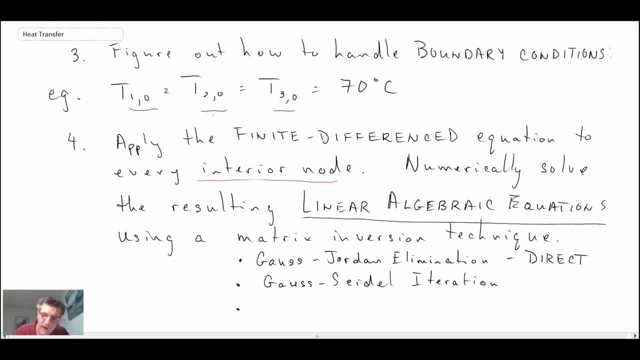 one requires iteration, a final one, and and then this is a code that hopefully I will be able to show you in two lectures from now, but it is using a Excel and that involves a circular reference and iteration. so those are different techniques that we can use to solve our set of linear 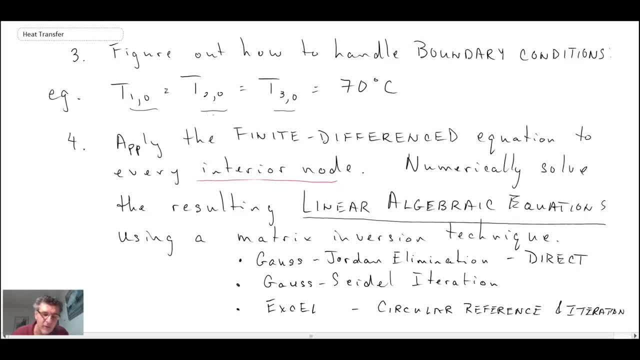 algebraic equations that result from each of the interior knows and applying the finite difference equation to them. And once we've done that, what will come out of that process? we will then obtain T M, N for all of the interior nodes. 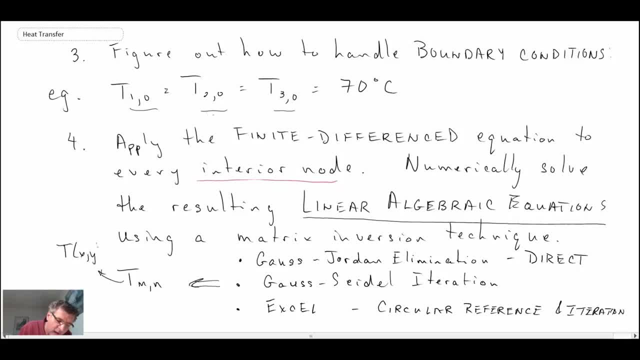 and that, essentially, is then giving us T, X, Y, where X and Y are at each of the discrete node locations that we established in the grid generation step at the beginning. So if you want finer resolution, make delta X and delta Y smaller. 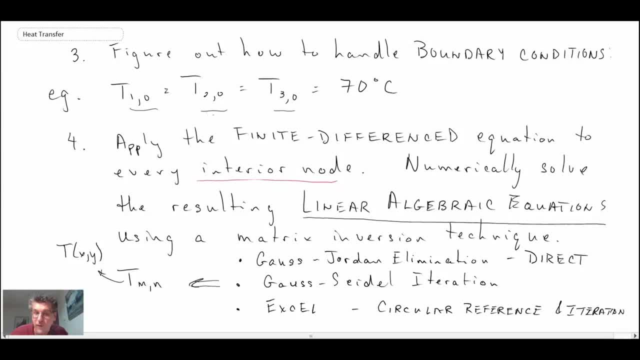 and you'll get finer resolution in your solution. But of course there'd be more points and it would take a little bit longer in terms of the numerical analysis. So that, in a nutshell, is kind of what the finite difference method applied to heat transfer looks like.